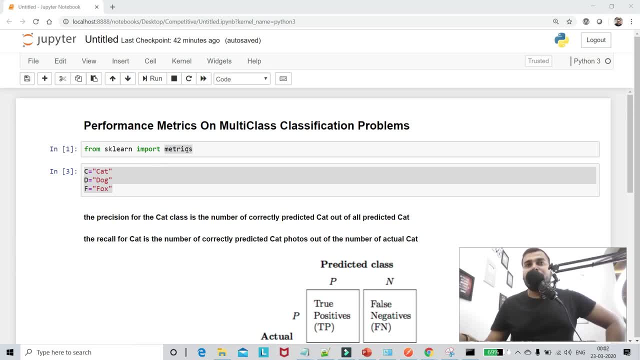 So here, what I'm going to do is that, first of all, I'm importing from a scale on import metrics, because a metrics- consider this library consists of, you know, classification reports, confusion, metrics, Classification reports is for precision and randomness, So I'm going to give you a very simple example. So here, what I'm going to do is 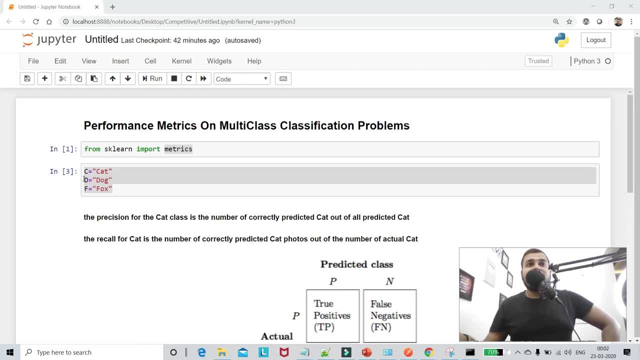 I'm going to give you a very simple example. So here, what I'm going to do is: I'm going to give you a very simple example. So here, what I'm going to do is call f1, score all that particular values. Now, what I'm going to do is that I'm going to consider 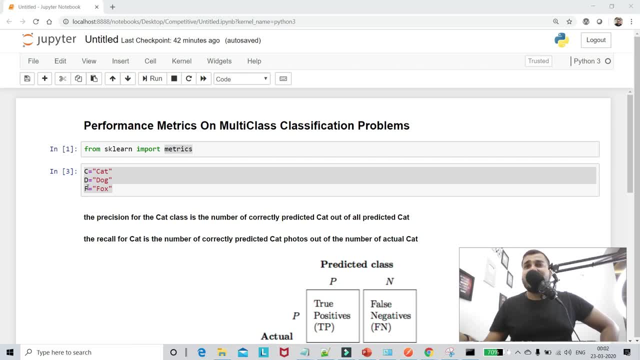 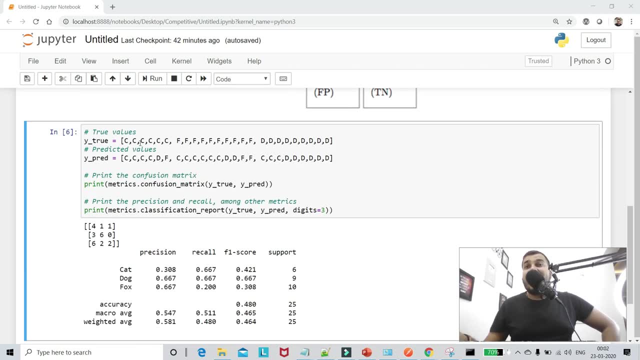 three categories: cat, dog and fox. So I have initialized this as constants. So I have in my variable c, b and f. Now what I'm going to do? I'm going to consider these are my output values, actual output values. Okay, why, true? So I have values like c, c, c, c, f, f, f, f, f, d, d, d, d d. 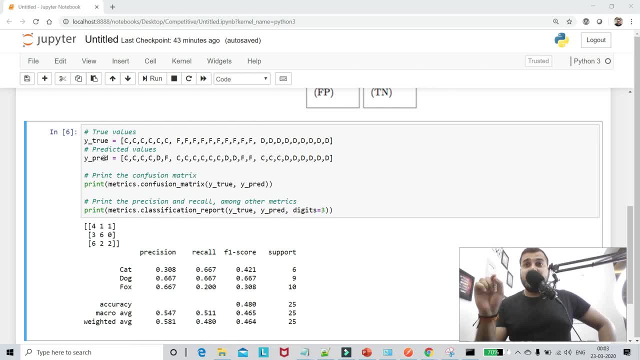 Okay, and then I'm not again developing any model. So here, consider that my model has predicted the values like y pred, c, c, c, c, d, f, These all values it has got predicted. Now I have my y, true. 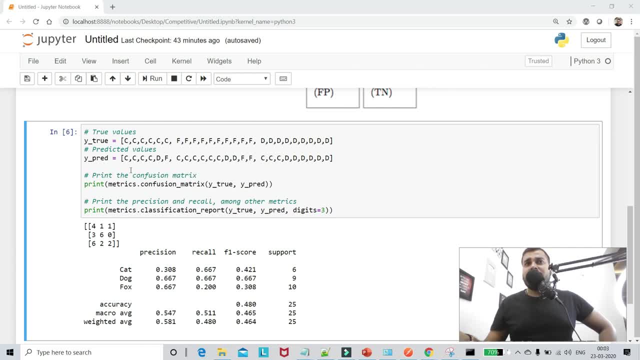 and this is my y predicted value. I'll try to find out the confusion matrix. In order to find out the confusion matrix, I have something called as metrics dot confusion underscore matrix. Here I'm going to give my value as y underscore true, y underscore pred. Now, when you give this usually for a binary, 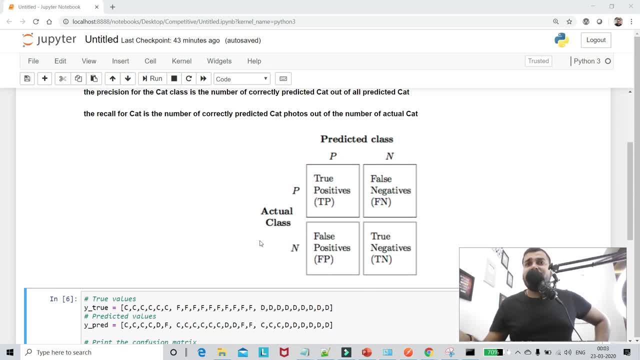 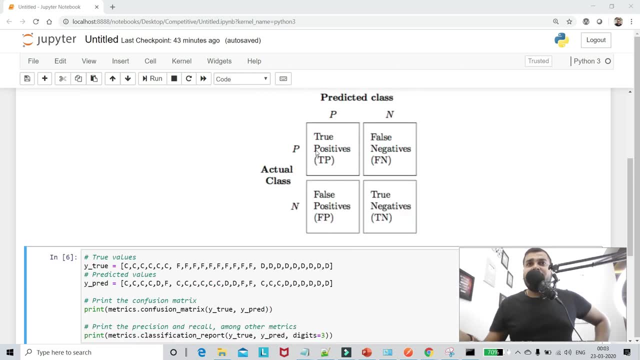 classification problem. I get this particular scenario. In my left hand side I have actual class which is just my positive and negative, My predicted class, positive and negative. Now in 3 cross 3 matrix you can see that I'll get my actual value over here. but I'll be having three records. Which three? 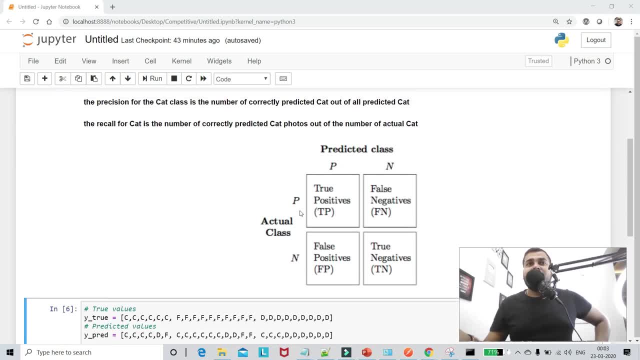 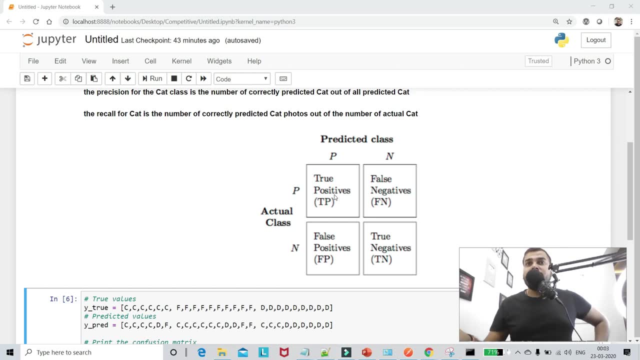 records: cat- Okay, the first one is cat, Cat, and the second record will be dogs and third records will be fox. Okay, actual values and if I go and see from the top, this will be my predicted values. Now, here you have all the values and again the column wise also. you'll be having three columns. 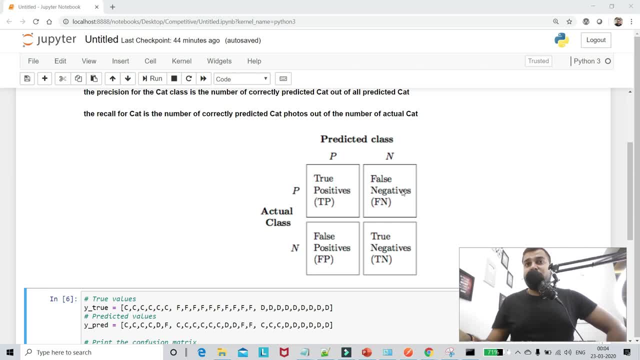 Okay, now you here. you have these terms like true positive, false negative, true, false positive and true negatives. Understand, guys, in multi-class classifications you cannot consider this kind of terms. Okay, so what we do is that if you want to calculate how, what will be the accuracy, you just have to see these diagonal elements, All the diagonal elements. 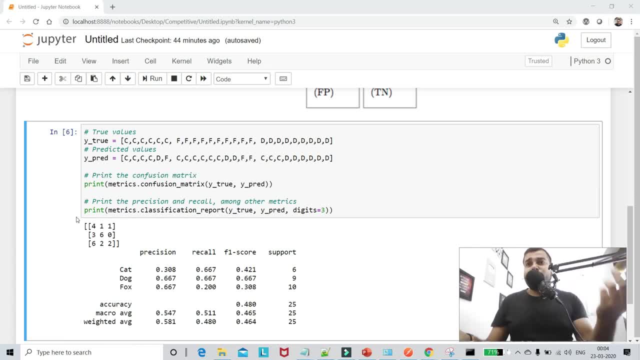 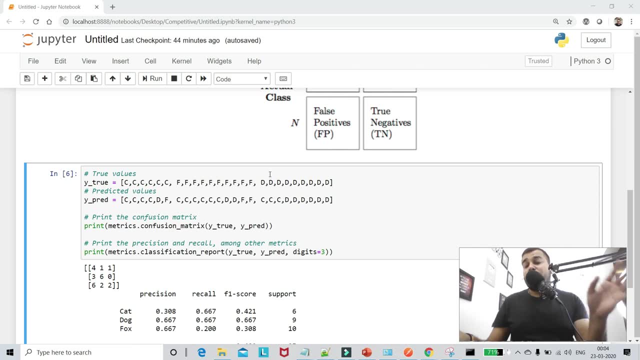 if you sum it up, divide by total sum of all the other elements will be actually your accuracy. Okay, but still we need to find out how we can actually recall with precision and how we can actually find out with respect to precision and recall. Now here I'm going to take some. 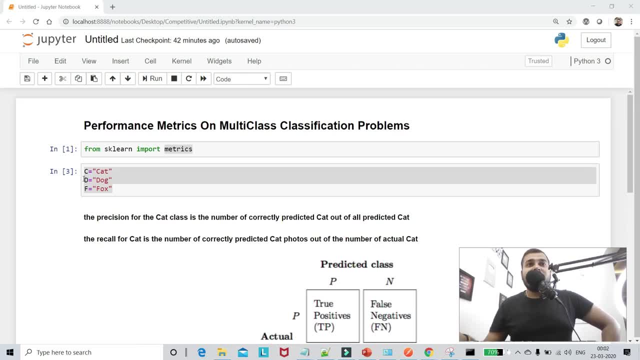 that first of all I'm importing from a scale on import metrics. So here what I'm going to do is call F1 score, all that particular values. Now what I'm going to do is that I'm going to consider three categories: cat, dog and fox. So I have initialized this as constants, So I have in my 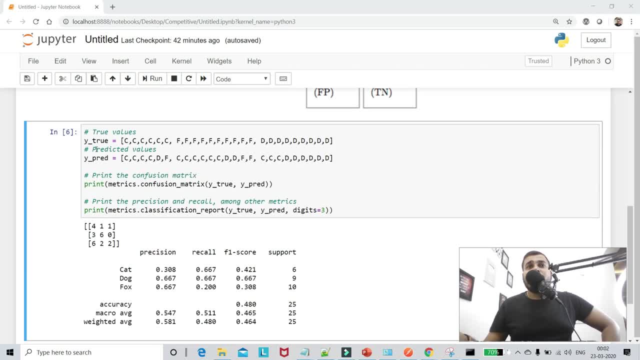 variable C, D and F. Now, what I'm going to do? I'm going to consider: these are my output values, actual output values. Okay, why? true? So I have values like C, C, C, C, F, F, F, F, F, F, D, D, D, D D. 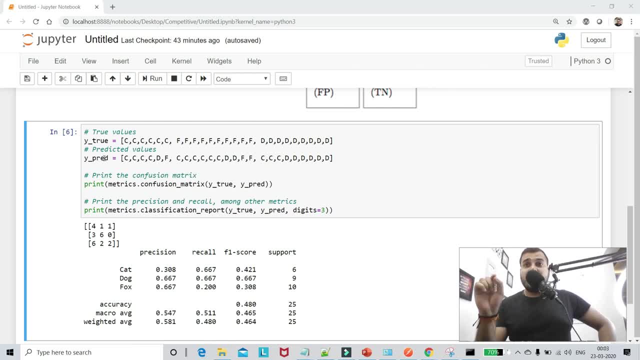 Okay, and then I'm not again developing any model. So here, consider that my model has predicted the values like wipe, red, C, C, C, C, D, F. These all values are going to be true, So I'm going to. 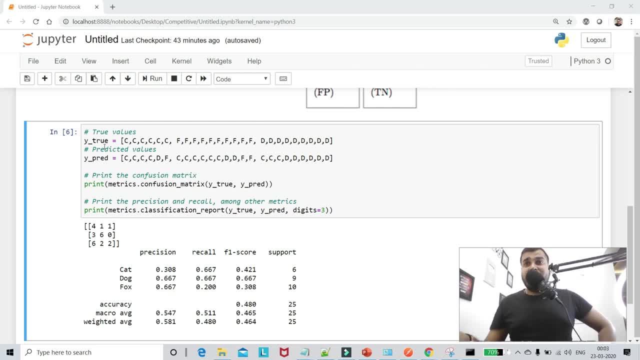 use it as got predicted. Now I have my Y true, and this is my Y predicted value. I'll try to find out the confusion matrix. In order to find out the confusion matrix, I have something called as matrix dot- confusion underscore matrix. Here I'm going to give my value as Y underscore- true Y. 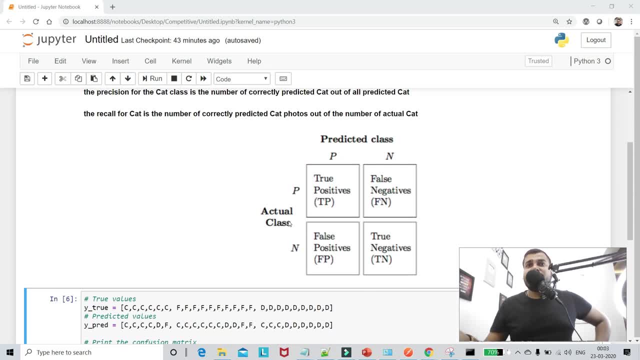 underscore right Now, when you give this, usually for a binary classification problem, I get this particular scenario. In my left hand side I have actual class which is just my positive and negative, My predicted class, positive and negative. Now in 3 cross 3 matrix you can see that I'll get. 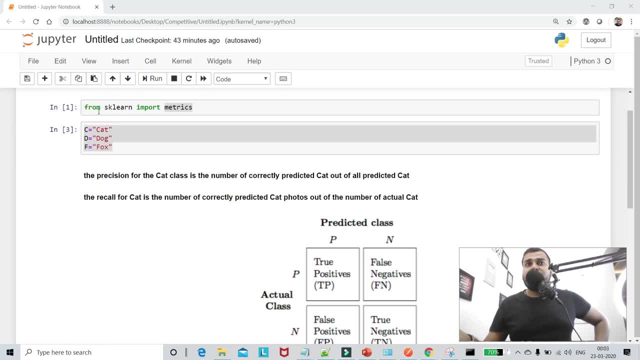 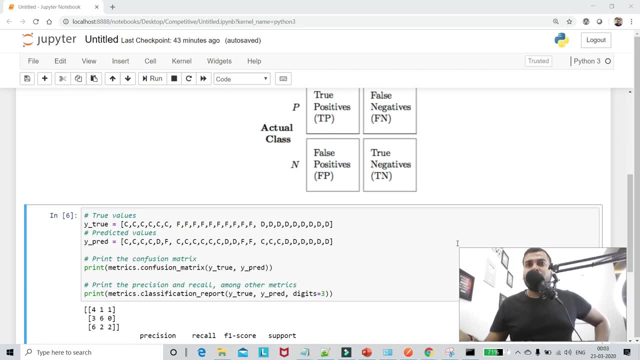 my actual value over here, but I'll have three records. Which three records? Cat, Okay, the first one is cat, Cat and the second record will be dogs and third record will be fox- Okay, actual values. And if I go and see from the top, this will: 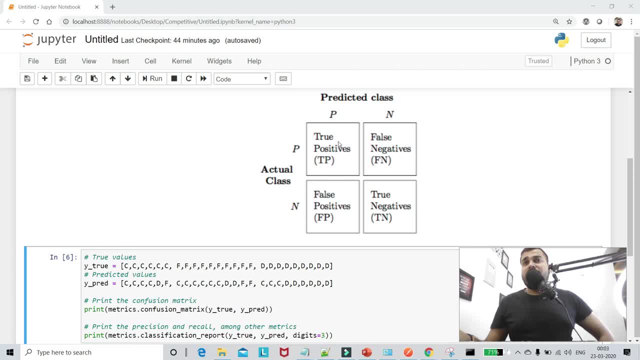 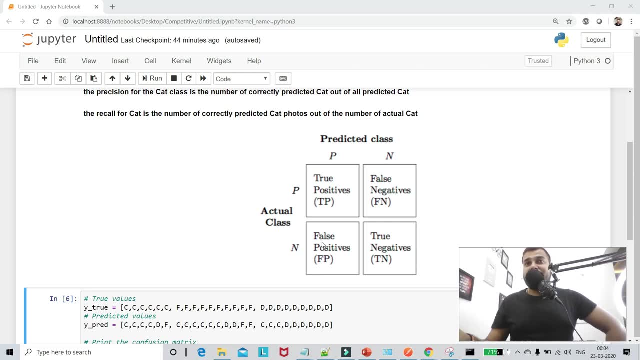 be my predicted values. Now, here you have all the values and again the column wise also, you'll be having three columns. Okay, now here you have these terms like true positive, false negative. true, false positive and true negative. Understand, guys, in multi-class classification you cannot consider. 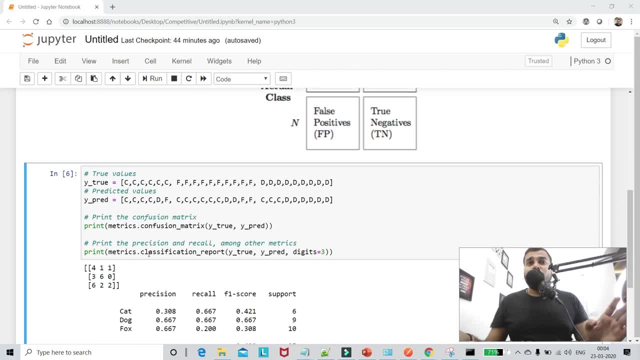 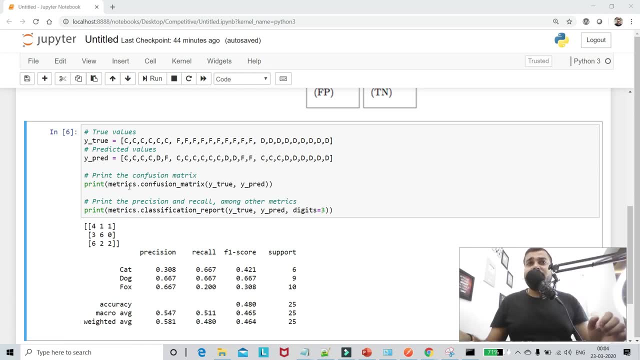 this kind of terms. Okay, Now, what we're going to do is that, if we what you want to calculate, what will be the equation? you just have to see these diagonal elements, All the diagonal items. if you sum it up, divide by total, some of all the other elements will actually be the accusation. Okay, 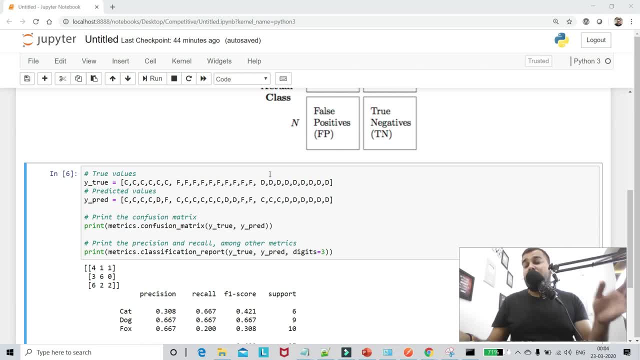 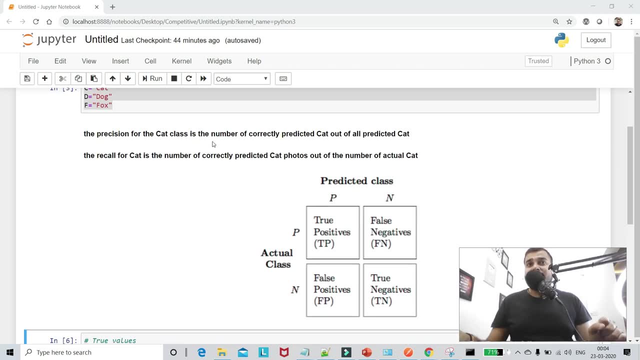 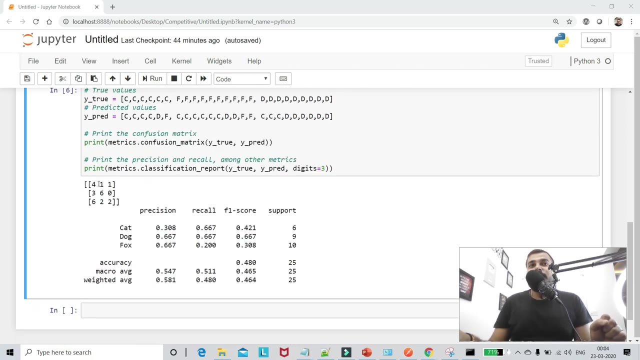 But still we need to find out that, how we can actually recall the precision and how we can actually find out with respect to precision in that class. Now, here I'm going to take an example of precision. Now for precision for cat-class, is the number of the predicted cat out of all the predicted cat? Now, first of all, we need to find out which is the actual. 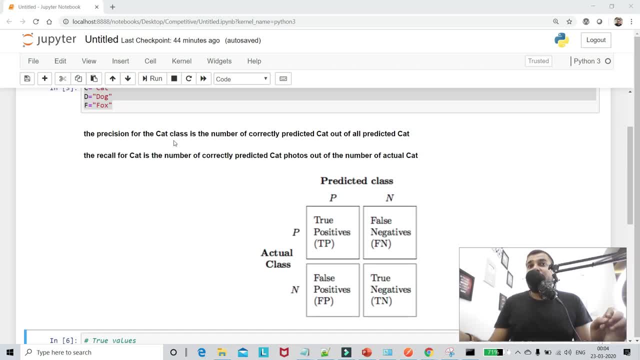 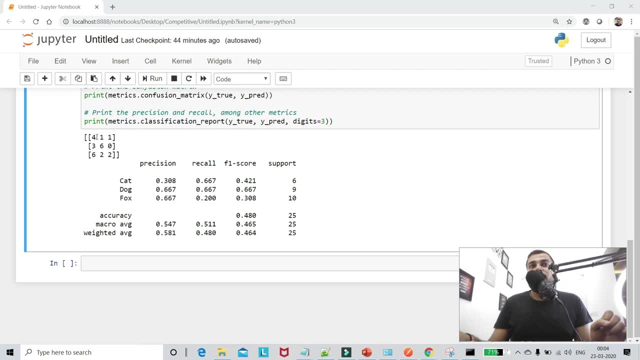 cat, okay. again i'm saying going to repeat: the precision for the cat class is the number of correctly predicted cat out of all the predicted cat. okay, so what is the correctly predicted cat? i can have four values, okay, but what about the all predicted cats? then i have to go and see my 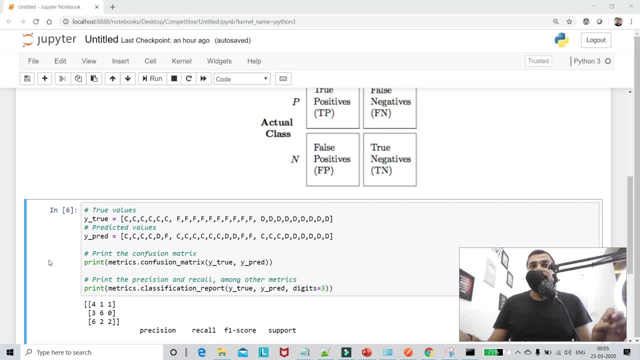 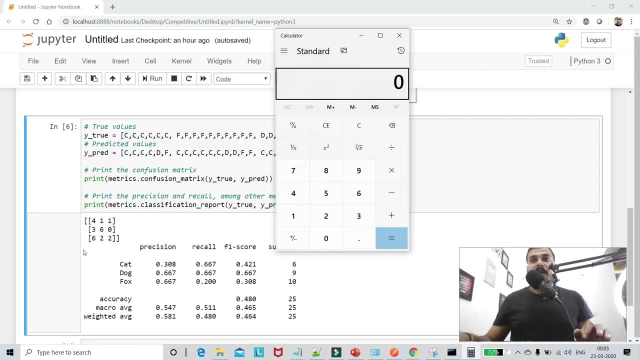 first column, whatever value comes in this particular column that i need to sum it up. so i have four, three, six. so if i go and open my calculator, okay, if i go and open my calculator and if i write, uh, four divided by which is my actual and our total predicted will be six plus. 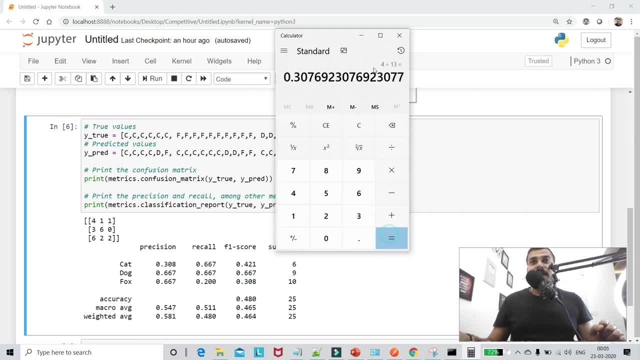 three, nine, nine plus four will be thirteen. so if i divide this particular value, i'm getting somewhere around 0.3076, which is nothing but 0.308. now, here you can see, for cat, the precision is this particular value. now it is pretty much simple and like this, only you calculate the. 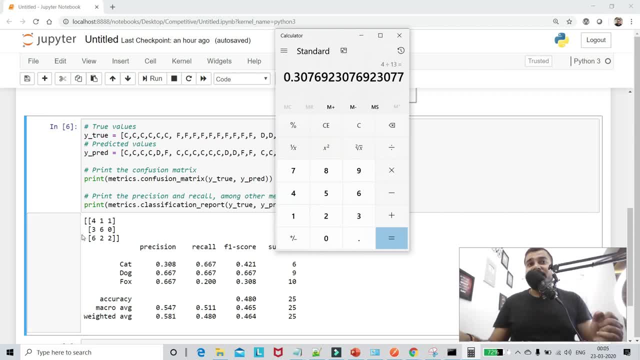 precision for all the other things right for dog. if you want to calculate again, my second column will- second row will be dog. dog basically represents this six value. so if i go and see what will be for dog, i can do six divided by nine. okay, so here you can see that 0.6667 i'm getting, which is absolutely. 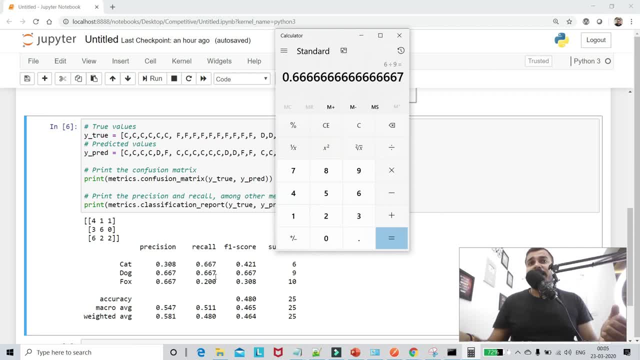 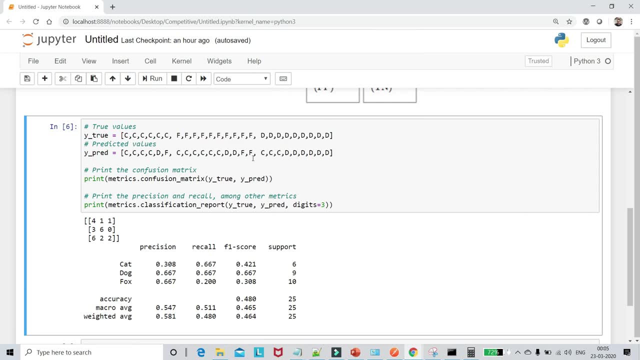 right and for the last, you can see that it will be two divided by three. then again, i'll be getting 0.667. now, this is how you actually calculate a precision. now, what is more important over here, guys, what is more important that you can actually see over here, is that how you are interpreting. 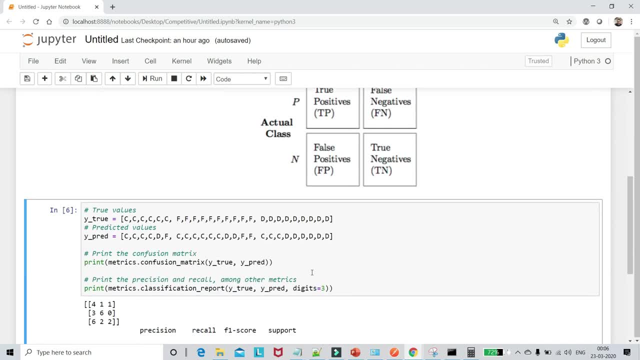 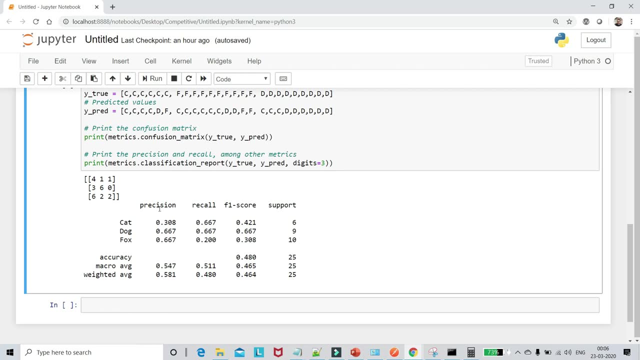 things everywhere. you cannot just find true, positive, false, negative. unless and until it is binary classification problem, you cannot go through this particular pattern. so it is very, very much important that how you represent this. now, for the cat, the precision is 0.308. for the dog, 0.667. for the fox, it is 0.667. now, the next important thing is that sometimes 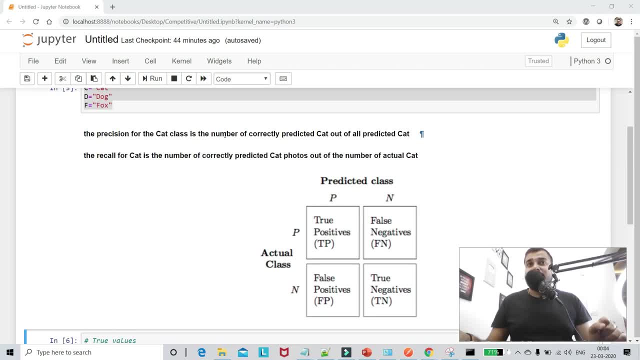 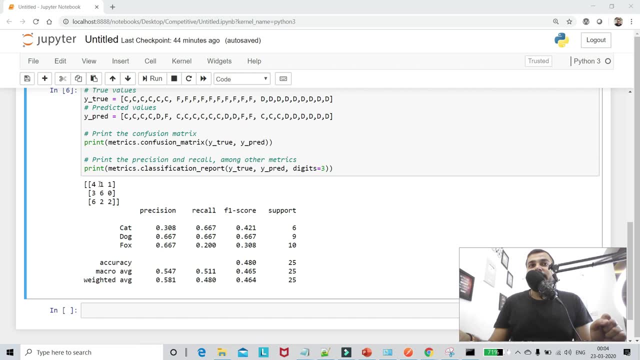 example of precision. Now for precision for cat class, is the number of correctly predicted cat Out of all the predicted cat? Now, first of all, we need to find out which is the actual predicted cat. Okay, again I'm saying, going to repeat, the precision for the cat class is the number of correctly 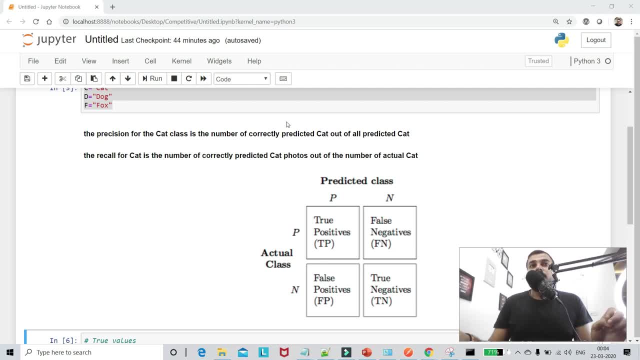 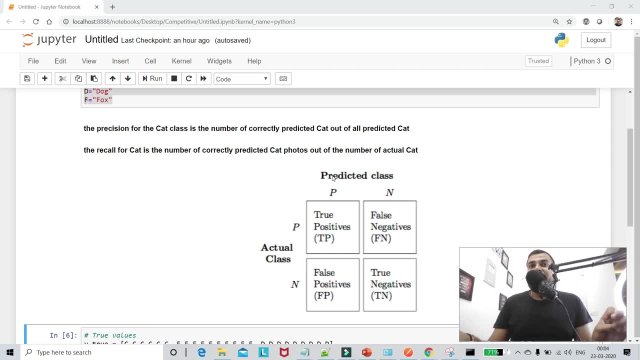 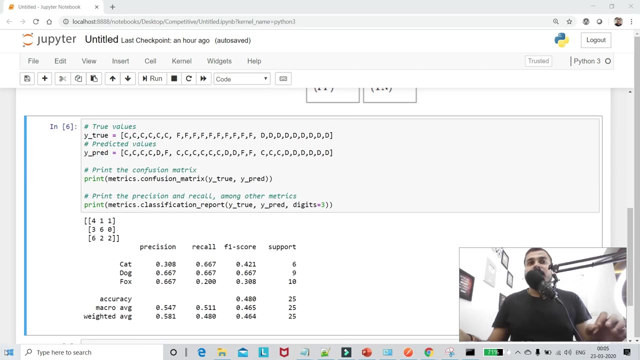 predicted cat out of all the predicted cat. Okay, so what is the correctly predicted cat? I can have four values. Okay, but what about the all predicted cats? Then I have to go and see my first column. whatever value comes in this particular column that I need to sum it up. So I have 4,, 3,, 6.. So if I 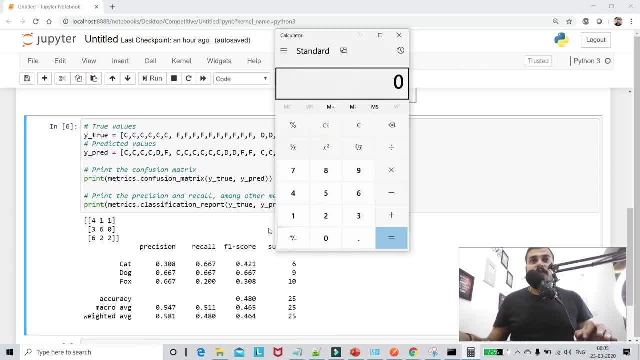 if I go and open my calculator and if I write 4 divided by which is my actual and our total, predicted will be 6 plus 3,, 9.. 9 plus 4 will be 13.. So if I divide this particular value, I'm getting 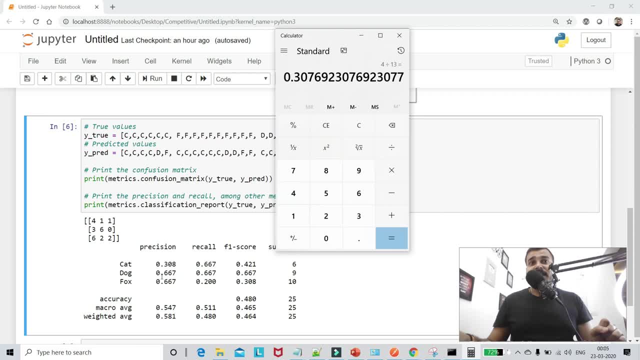 somewhere around 0.3076, which is nothing but 0.308.. Now here you can see. for cat, the precision is this particular value. Now, it is pretty much simple and like this, only you calculate the precision for all the other things. right, For dog, if you want to calculate again, my second column. 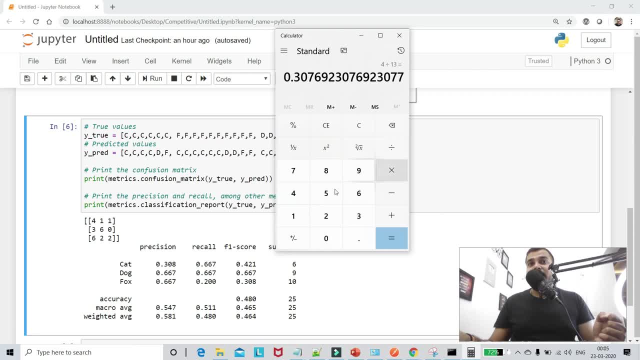 second row will be dog. Dog basically represents this 6 value. So if I go and see what will be for dog, I can do 6 divided by 9.. Okay, so here you can see that 0.6667 I'm getting, which is absolutely right, and for the last, you can see that it will be 2 divided. 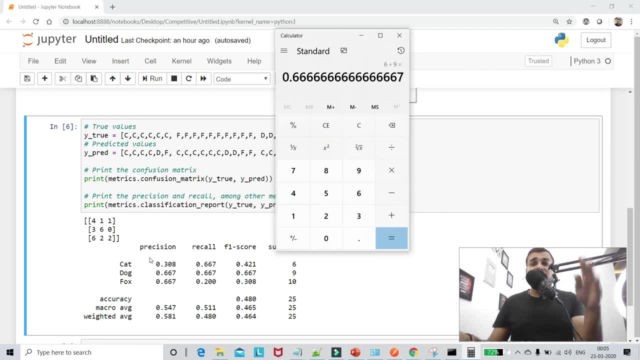 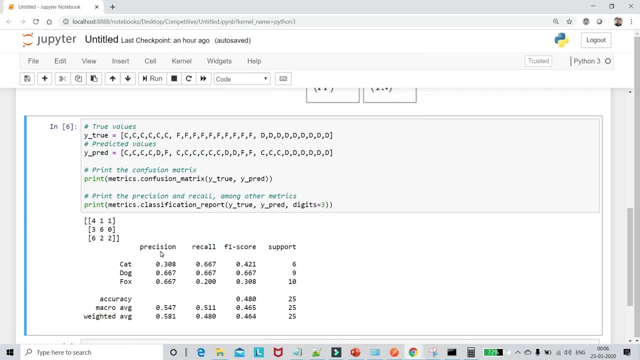 by 3, then again I'll be getting 0.667.. Now, this is how you actually calculate a precision. Now, what is more important over here, guys, What is more important that you can actually see over here, is that how you are interpreting things. Everywhere you cannot just find true positive, false, negative. 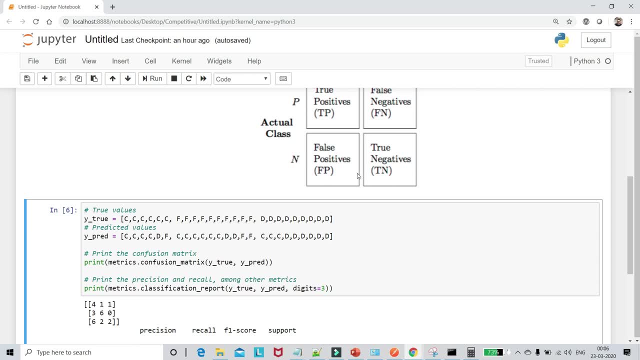 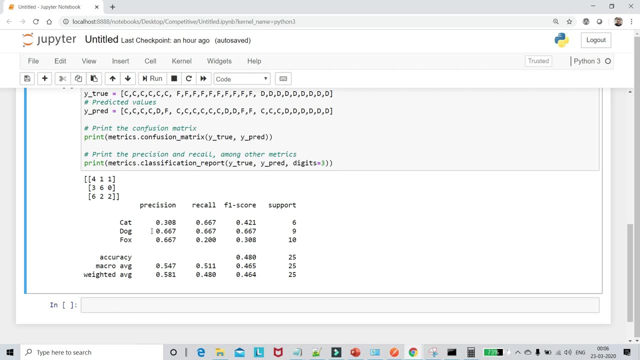 unless and until it is a binary classification problem, You cannot go through this particular pattern. So it is very, very much important that how you represent this. Now, for the cat, the precision is 0.308.. For the dog, 0.667.. For the fox it is 0.667.. 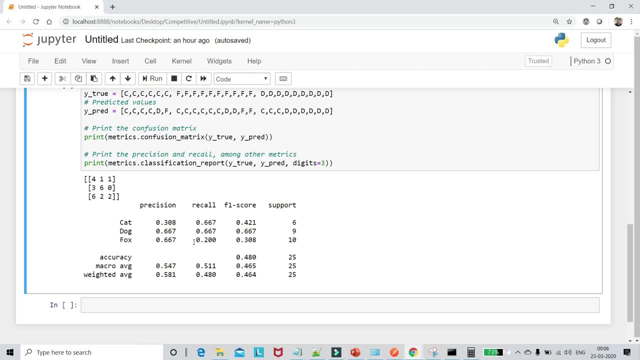 Now the next important thing is that sometimes- I say that for a particular use case- you also have to need to determine, if you're going to implement F1 score, whether the false positive is important or false negative is important. Over here again: the false positive and false.